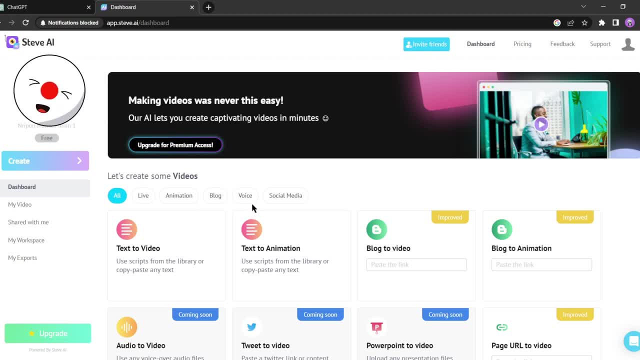 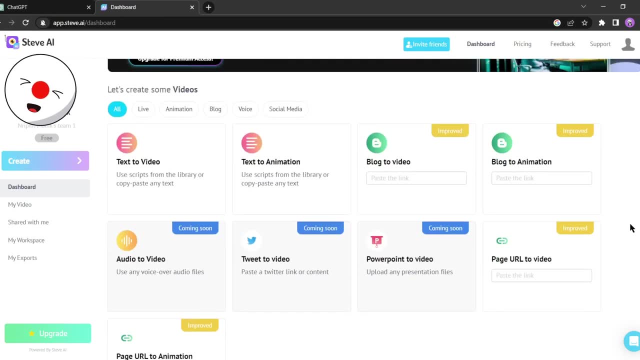 There are several option available here: text-to-video, text-to-animation, blog-to-video, blog-to-animation, audio-to-video, tweet-to-video and many more. It's really a very, very cool video generation AI, But today we will make animation video, So I am clicking on. 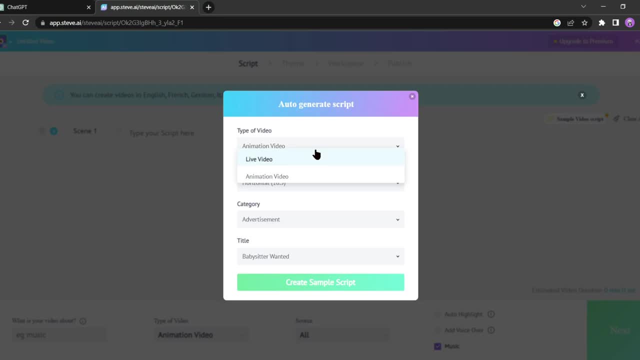 text-to-animation. Now select your video type. I am selecting animation. Then select video ratio. For YouTube video, always select 69.. After that, select video category and your video title. Once you've done that, click on create sample script. Steve AI will generate a sample script based on your story. But before we proceed, 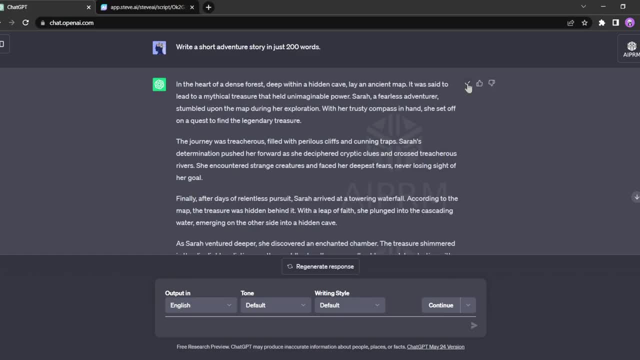 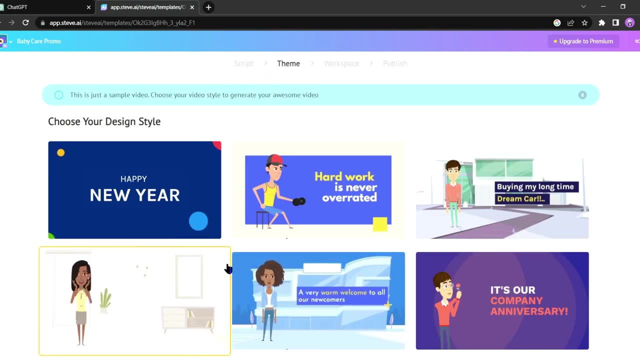 let's clear out their sample script. Now let's head back to chat GPT. copy our adventure story and paste it into Steve AI Great. Click next to continue. Now you have to select a template. Now AI will generate visual and story board for us. 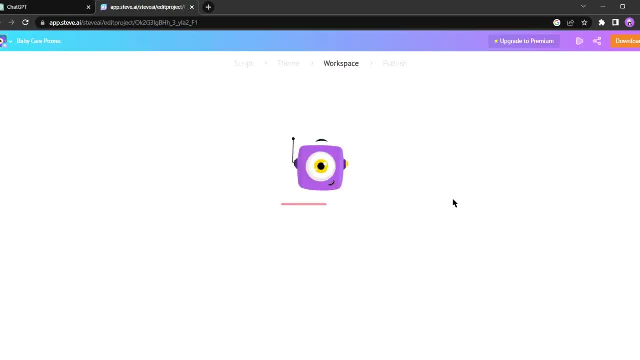 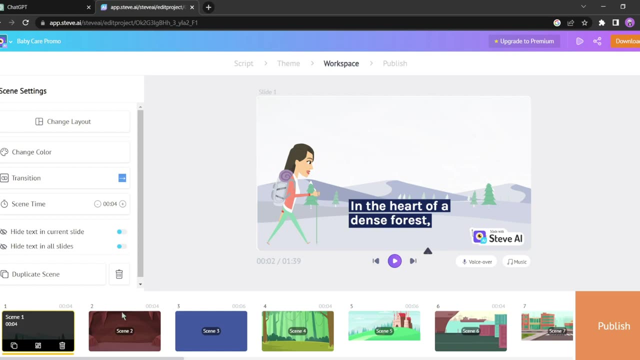 It will take some time. Let's fast forward this part. Fantastic Steve AI has generated scenes for our script. Now it's essential to review each scene carefully and make any necessary changes. Let's go through this together. In the very first scene, we will change the background. First, click on the background. 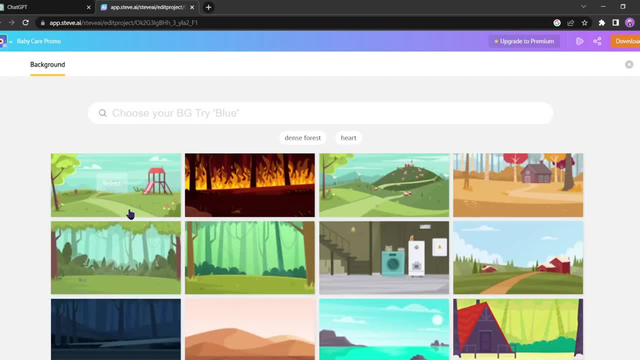 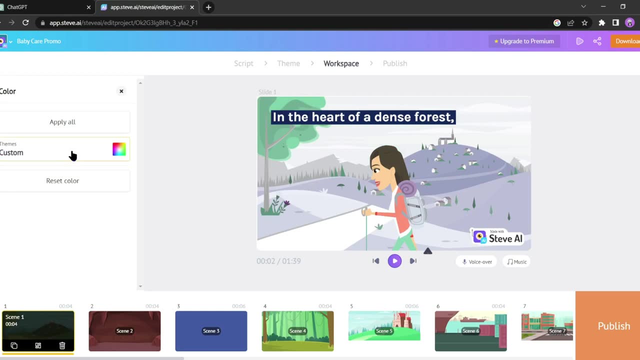 footage and then click on change background here. Select one of them which is best choice for your video. Next, change the background color. I am resetting the color as I want the original green backdrop In scene 2, our context mentions an ancient map, but the footage isn't relevant to. 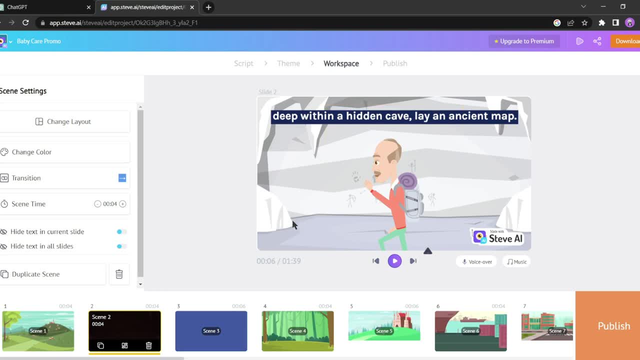 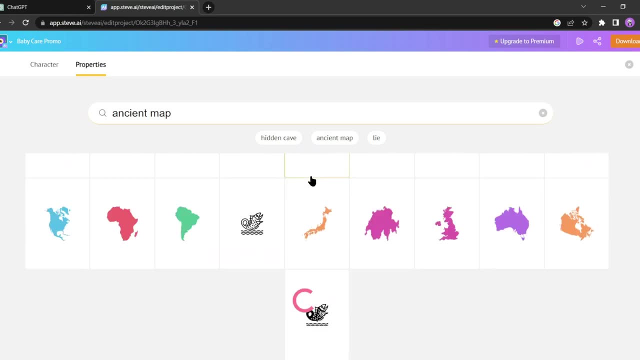 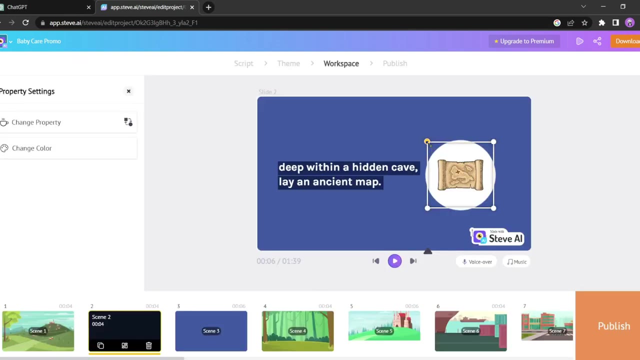 our video. Let's change that. Click on the avatar, then select, change character. click on property and choose ancient map. steve ai offers a wide variety of maps to choose from, so pick the perfect one for your story. i am selecting this one. remember to review all the 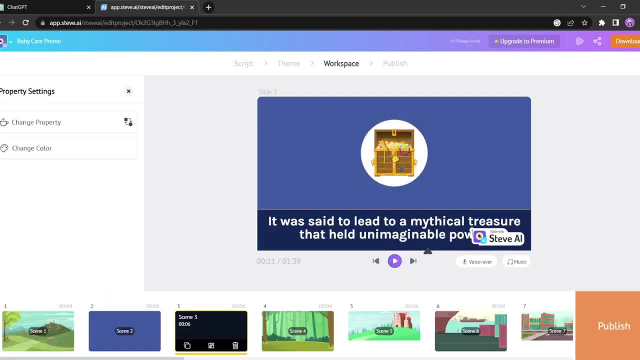 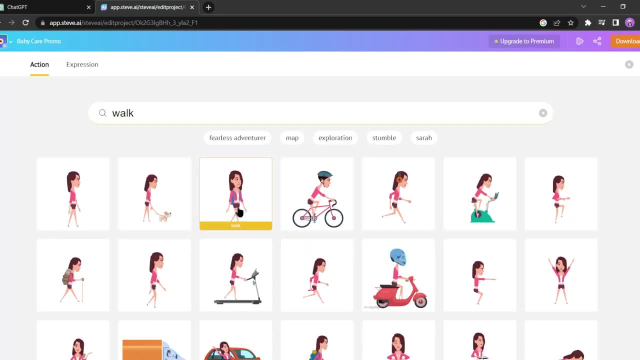 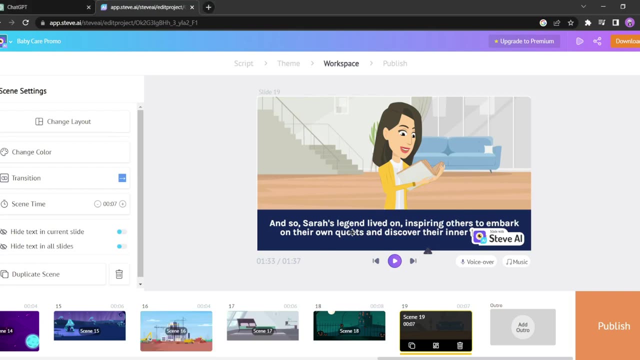 scenes and make necessary changes where needed. i'll fast forward through this part for time saving purposes, but i strongly recommend dedicating enough time to editing. quality editing is crucial to leaving a positive impression on your audience, so give proper time on editing. excellent. we've completed the visual editing. now it's time to add a voiceover. 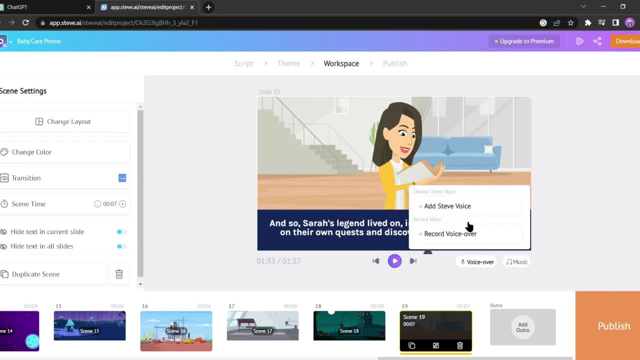 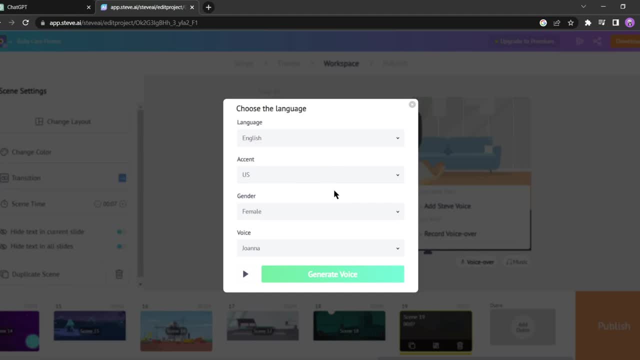 to our video. you can either record your own voice or use steve ai's voice generation feature. for this video, i'll use steve ai's voice. now select your desired language, accent and gender for the voiceover. steve ai offers various voice models to choose from. i'll go with joanna for. 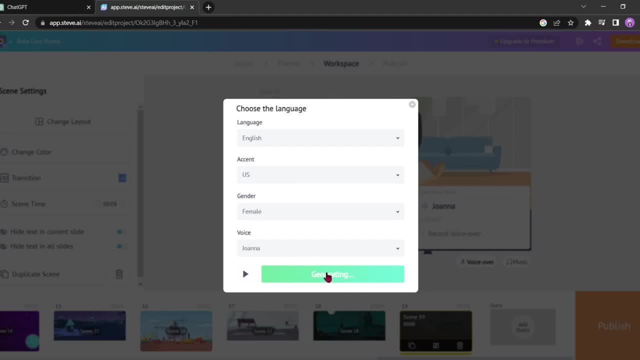 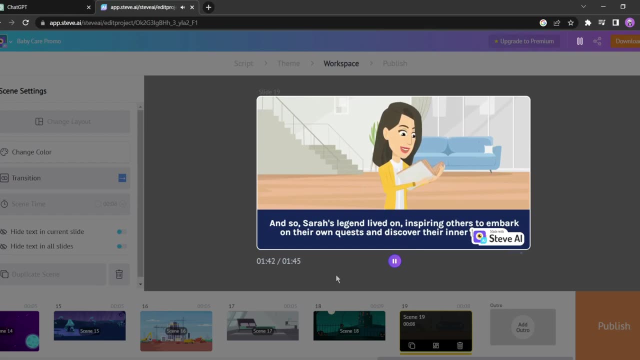 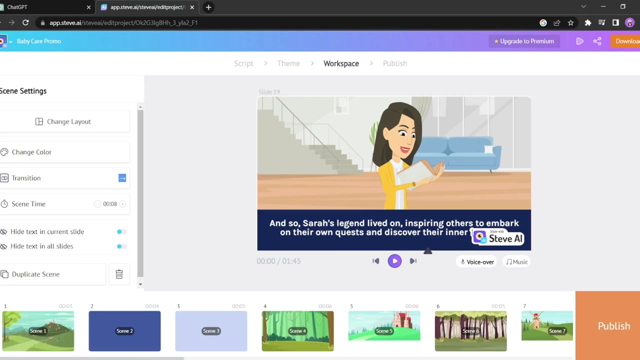 this video. all right, let's click on generate. let's play the video to check our voiceover. and so sarah's legend lived on, inspiring others to embark on their own quests and discover their inner strength. wow, it sounds incredibly natural. steve ai does a fantastic job. 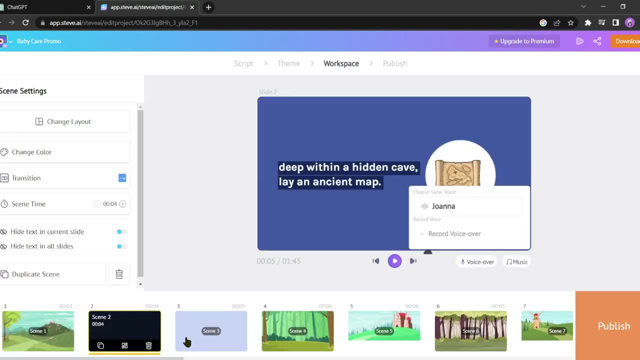 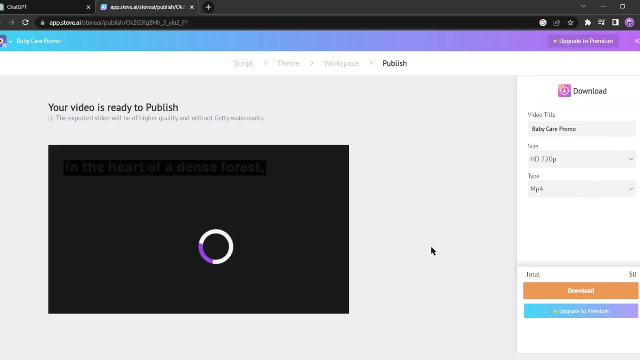 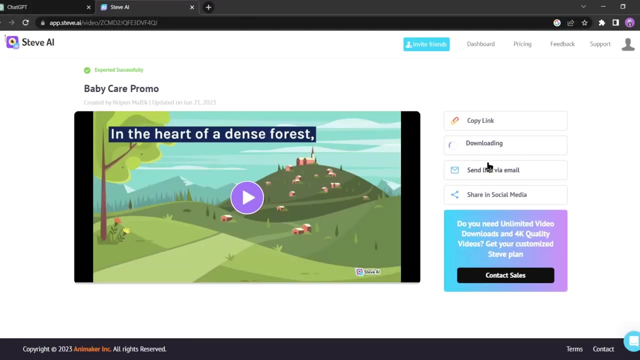 with voice generation. now that everything is set, it's time to publish our video. click on publish and steve ai will start processing the video. once it's done, you can download it. let's fast forward through the rendering process. okay, our video is now ready. click on download. here we have successfully created our animation video. let's play the video. 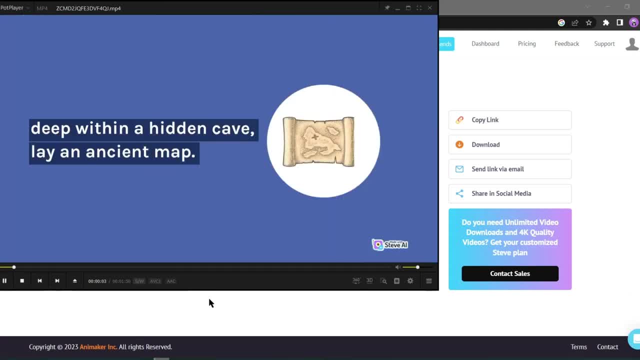 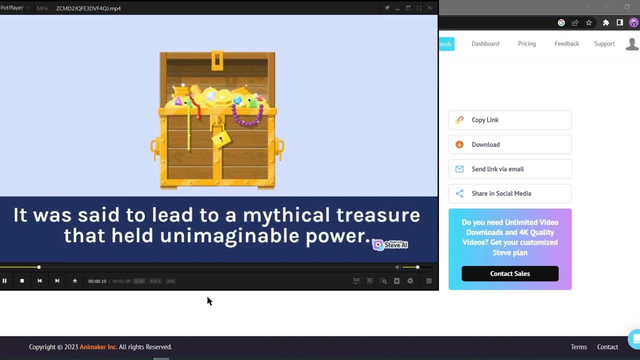 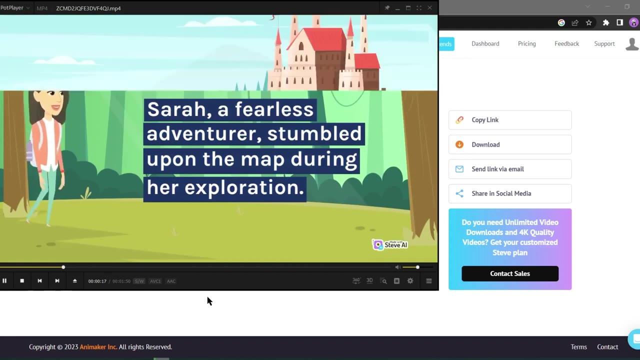 in the heart of a dense forest, deep within a hidden cave lay an ancient map. it was said to lead to a mythical treasure that held unimaginable power. sarah, a fearless adventurer, stumbled upon the map during her exploration. with her trusty compass in hand, she set off on a quest to find. 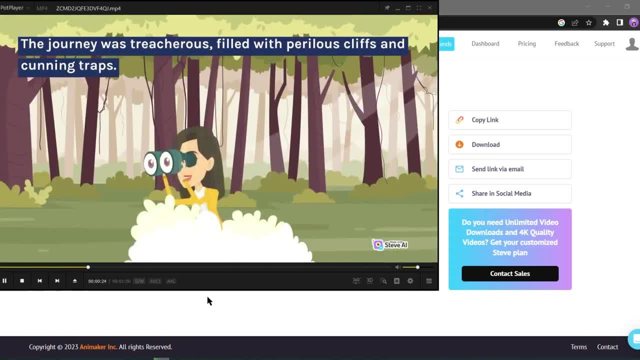 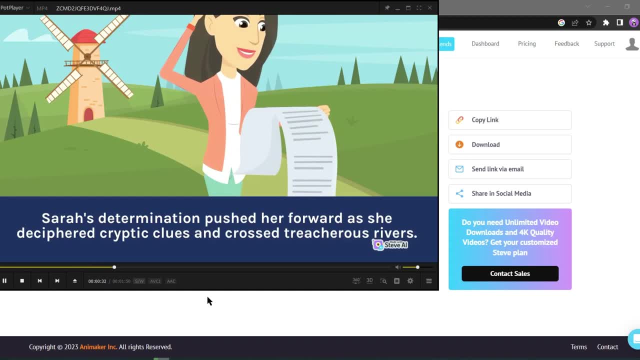 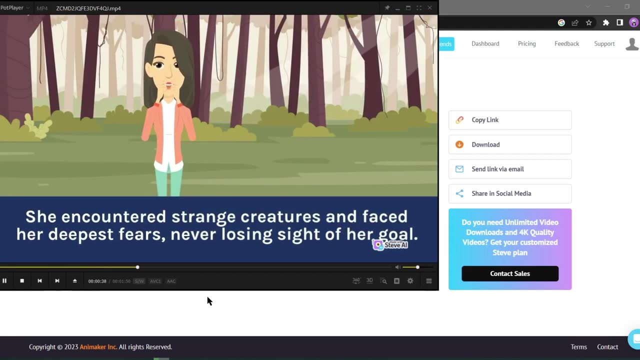 the legendary treasure. the journey was treacherous, filled with perilous cliffs and cunning traps. sarah's determination pushed her forward as she deciphered cryptic clues and crossed treacherous rivers. she encountered strange creatures and faced her deepest fears, never losing sight of her goal. finally, after days of relentless pursuit, sarah arrived at 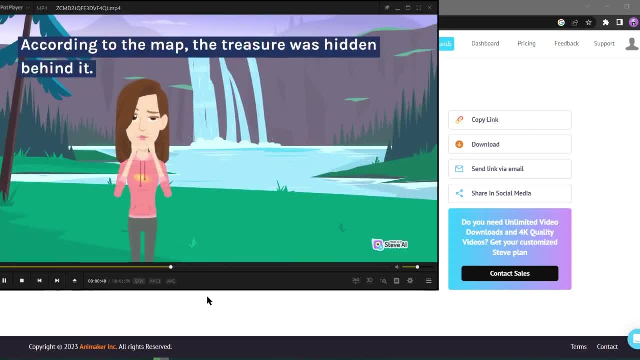 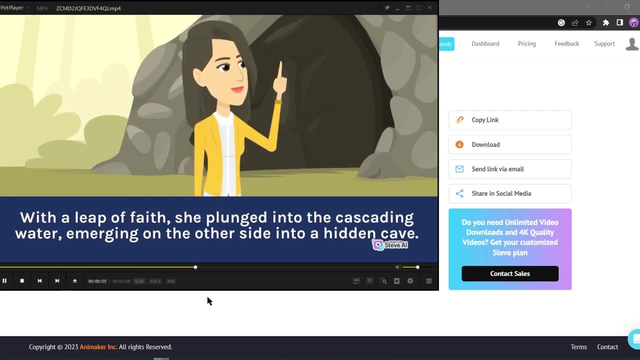 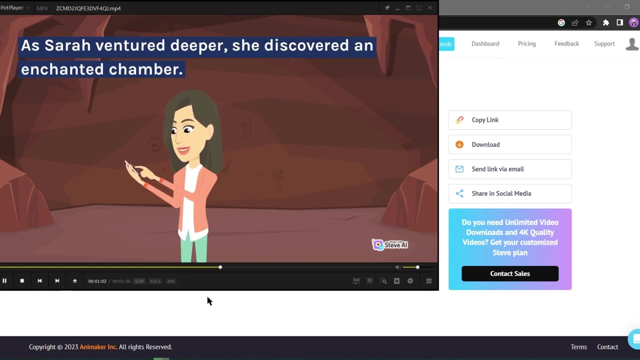 a towering waterfall. according to the map, the treasure was hidden behind it. with a leap of faith, she plunged into the cascading water emerging on the other side into a hidden cave. as sarah ventured deeper, she discovered an enchanted chamber. the treasure shimmered in the dim light radiating in otherworldly glow.